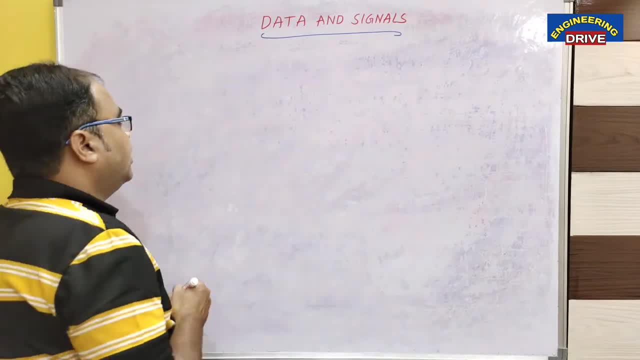 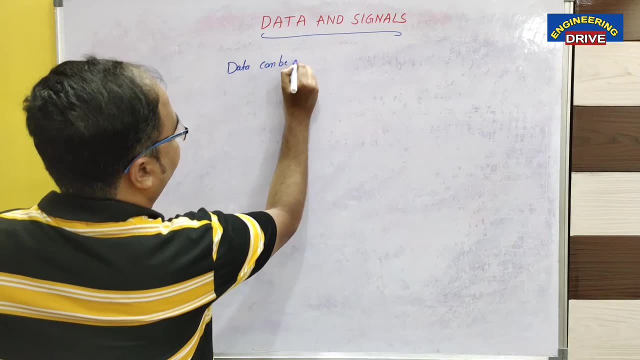 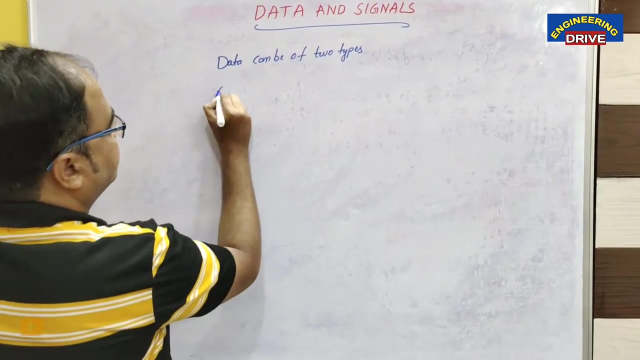 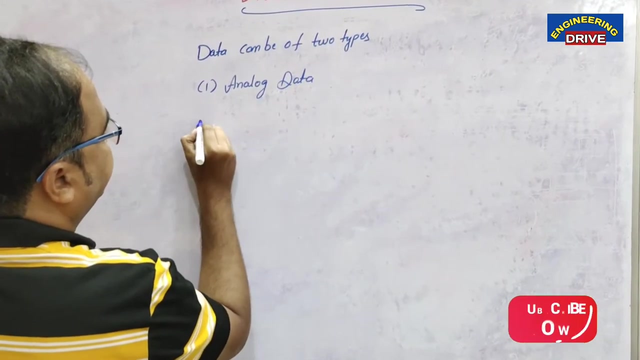 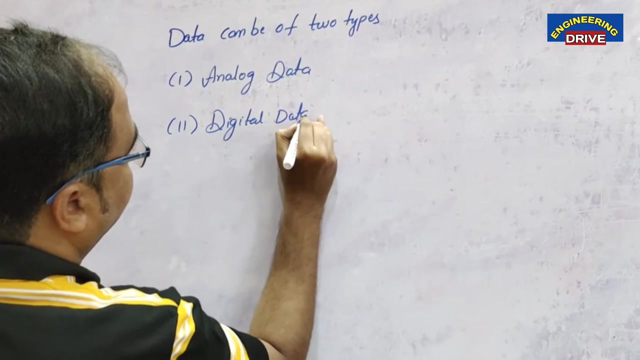 layer of the OSI reference model. So, dear students, data can be of two types. Data can be of two types. One is analog data and the second type of data is a digital data. So we need to remember these two names When we are talking about. 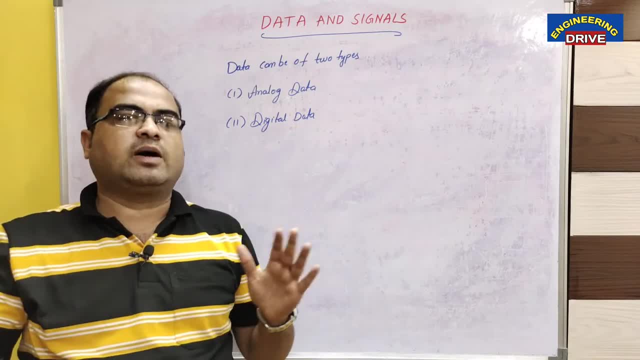 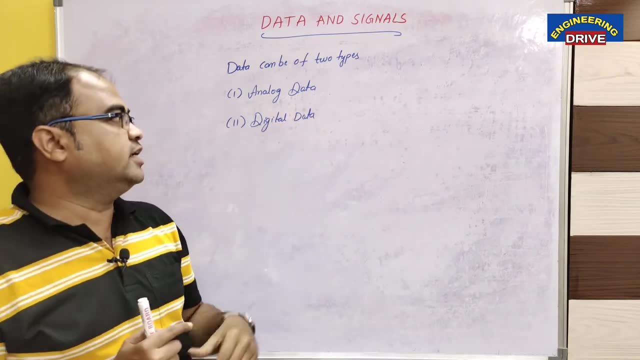 network, when we are talking about physical layer, when we are talking about the communication mechanism, we need to know in networks that there are two types of data. One is analog data, another one is digital data. So what is actually analog data? Analog data refers: 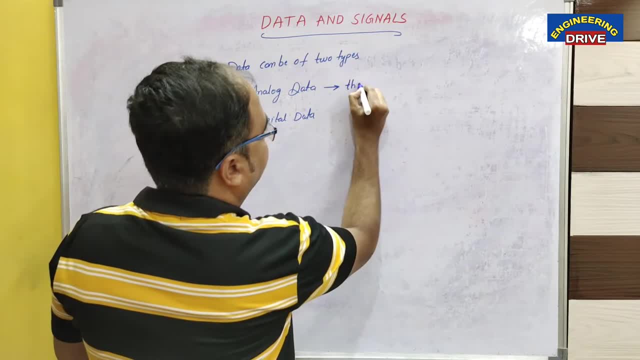 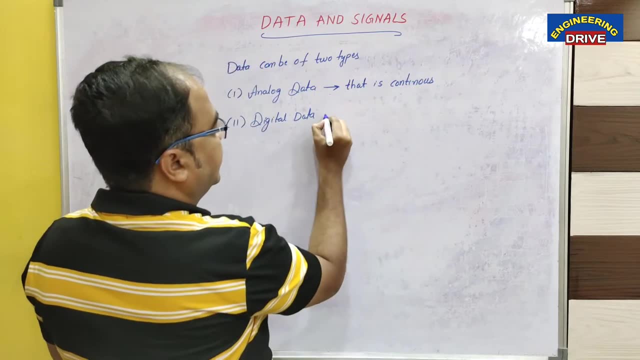 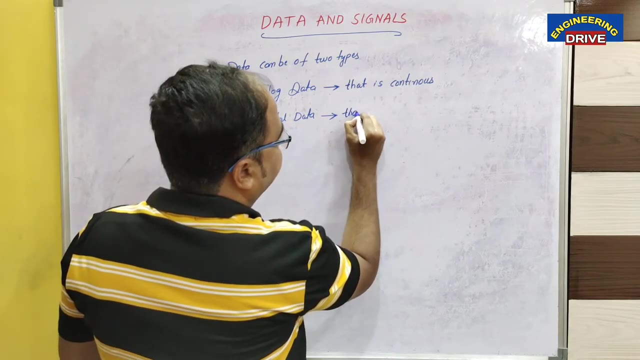 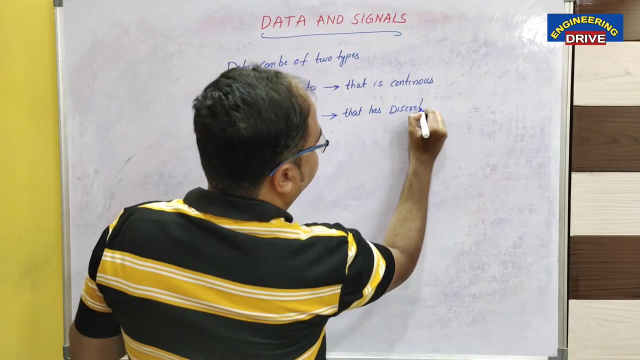 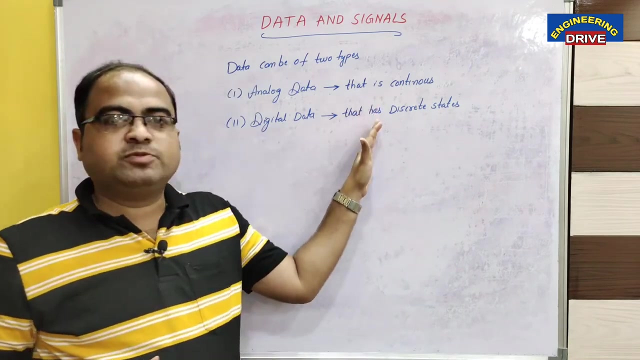 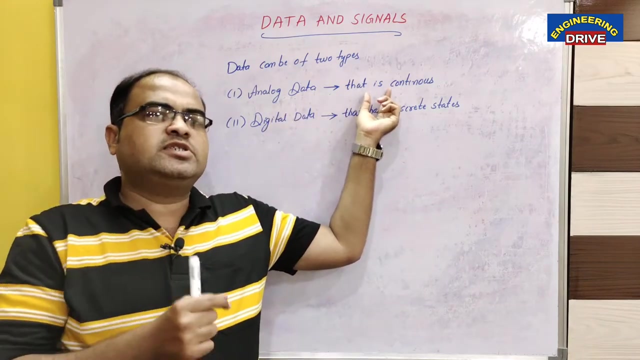 to the information that is signal, Whereas a digital data is nothing but which refers to the information that has discrete states. Now, this is the main difference between a analog data and digital data. Next, I will give an example also to you. analog data is nothing but if something which is. 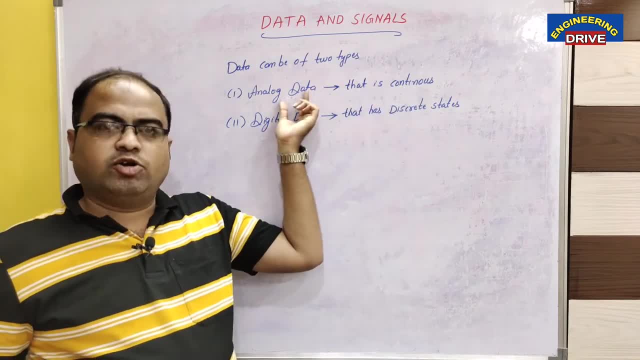 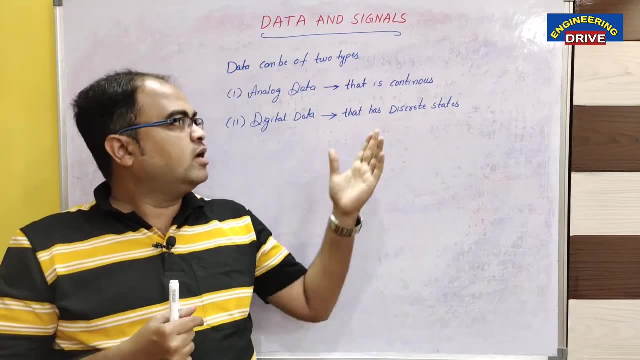 continuous form of information, then we can say that it is analog data. And if we, instead of continuous, if the data is in different states, if the data is in a non-continuous manner, then we can talk about that data as a digital data. 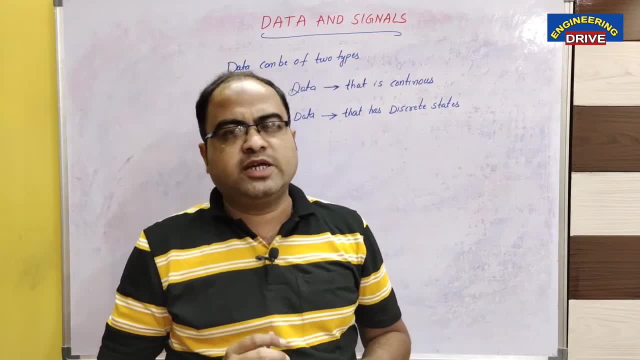 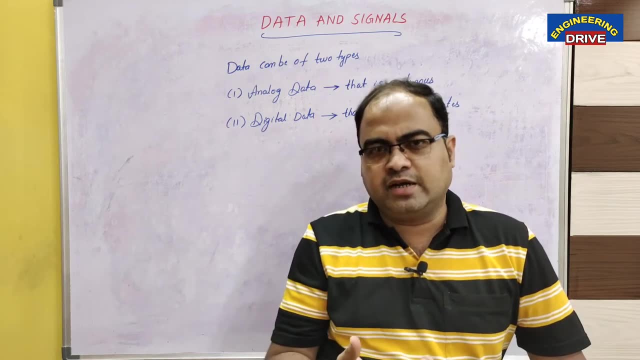 Now, sir, can you give an example of what is analog data, sir? So, dear students, now I can give one best example for to all of you for analog data. Like I am speaking here now, I am speaking continuously some type of topics here, like today I am. 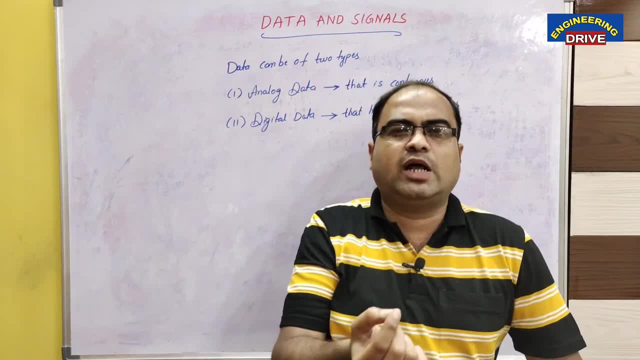 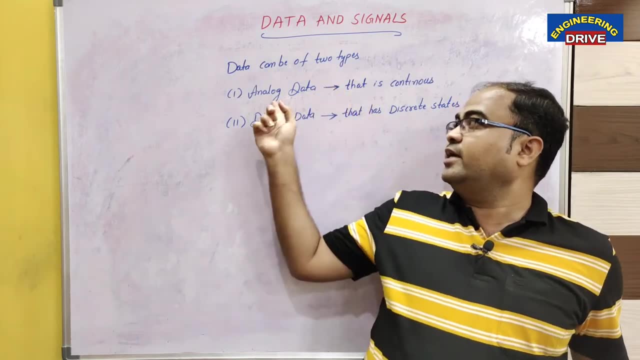 discussing about what is data and signals. So, non-stop way, with a small pauses, I am speaking here. is it right or not? So this type of speech, this type of lecture, we can take it as an example of analog data, Because what type of data is analog? data which is continuous or that is continuous? 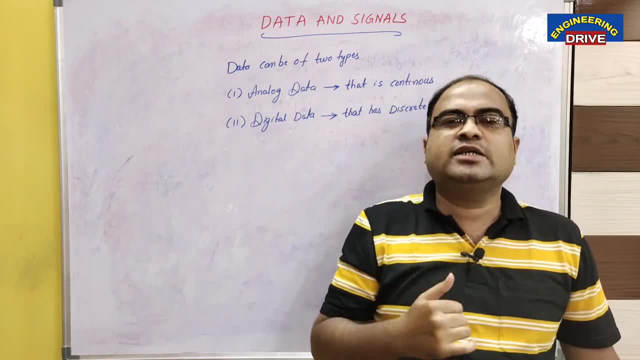 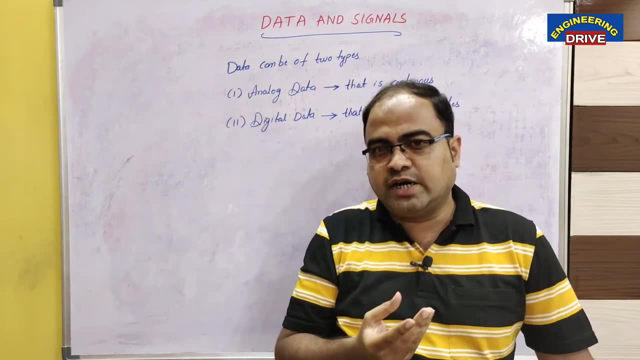 form of data is analog data, So whatever I am speaking, it is in continuous form. Now, whenever I am speaking, this is an example of analog data. Now, who is capturing my analog data? you know this microphone, this microphone, this mic. 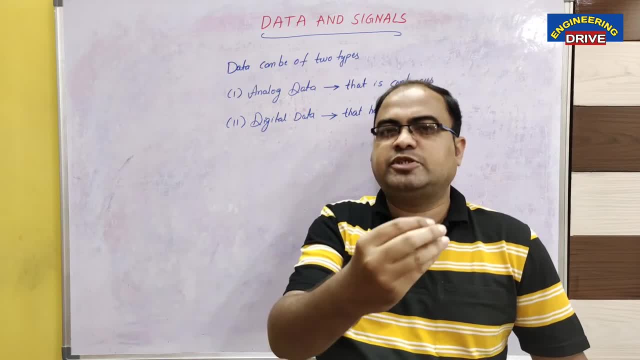 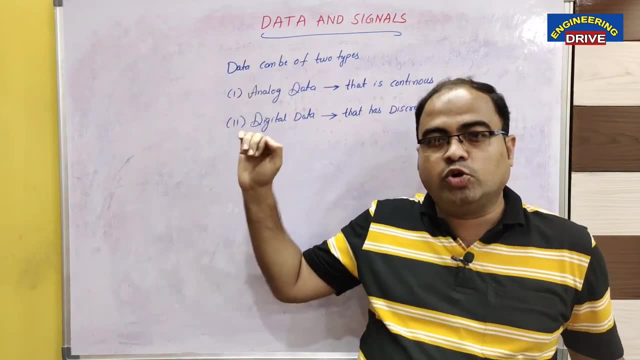 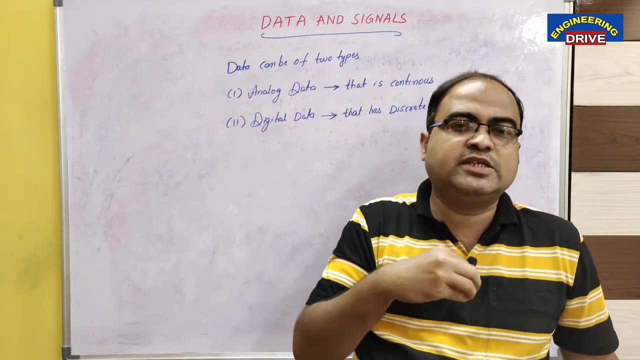 which is there on my t-shirts collar. it is capturing that analog data. that is my voice. And what my microphone is doing: it is converting this analog data into a signal. we call the signal as analog signal. analog signal, So something which is outside is analog data. 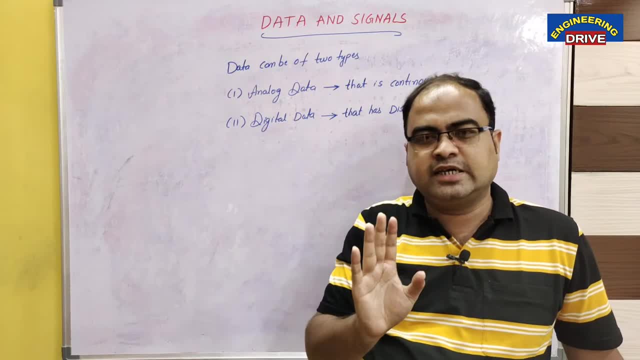 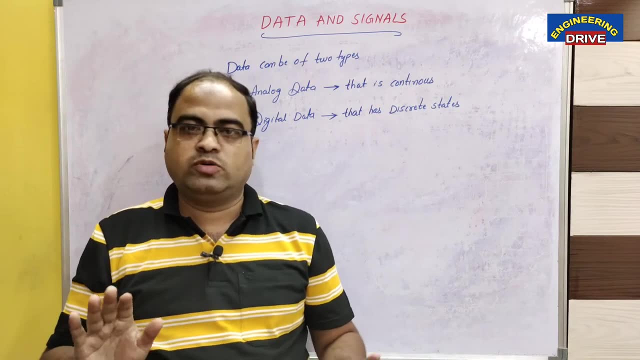 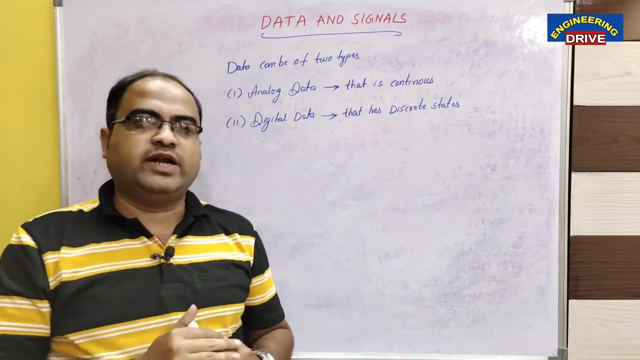 Something which is inside is analog signal. Is it clear Now, sir, whether computers understands the analog data or analog signal? sir, The answer is no. computers does not understand the analog data or even analog signals. Computer understands only one type of data, that is, digital data. computer understands. 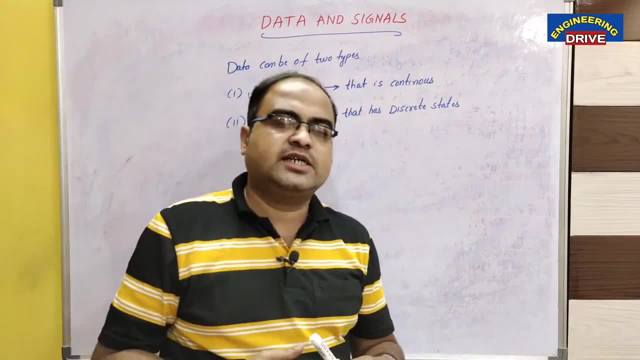 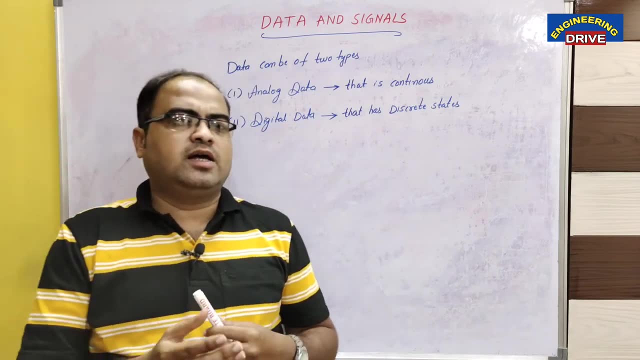 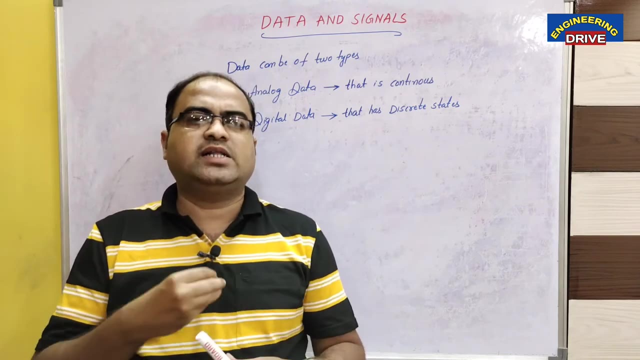 only digital data. Now, what type of data is digital data, sir? We understood analog data example. can you give an example of digital data? So, dear students, the files that we have that we will store in our computers memory, the data or video files, audio files, document files which we will store in our mobile phones. 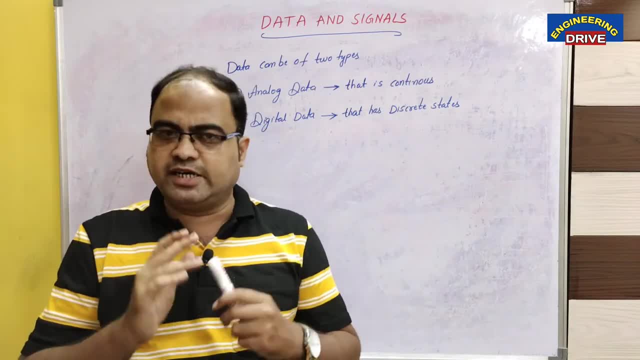 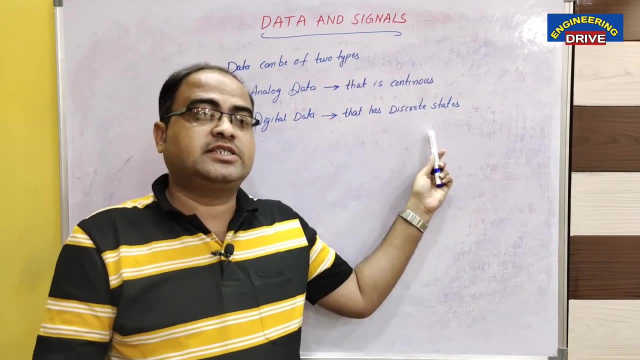 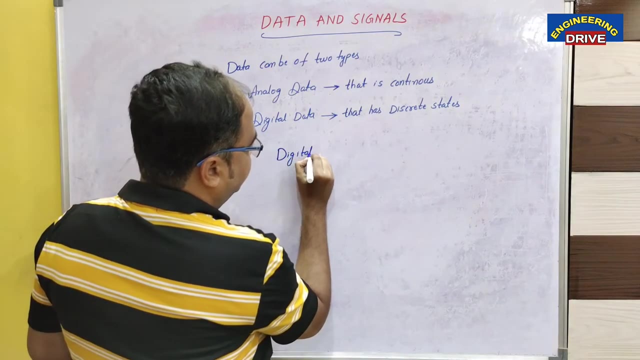 memory, smartphones memory. they are all examples of digital data. Is it right Now digital data? why we are calling that digital data is nothing but which is having discrete states, Because the digital data will be available in only digital data. Okay. 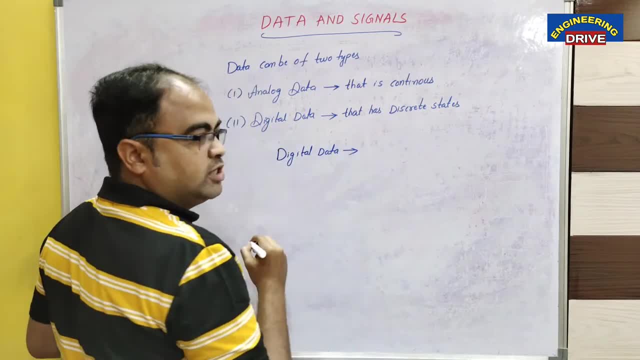 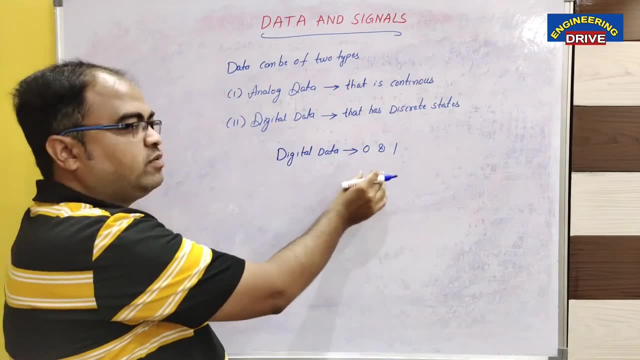 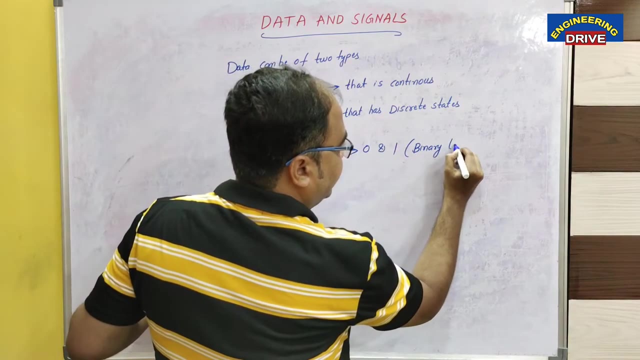 The digital data will be available by using two types of digits. What are those? 0 and 1.. Okay, What we call the language which our computer makes use of to store zeros and ones. we call this language as binary language. binary language. 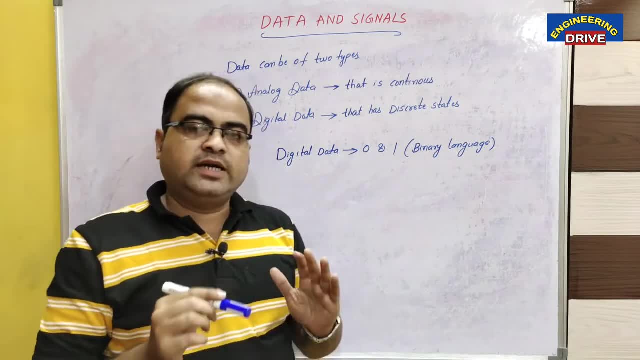 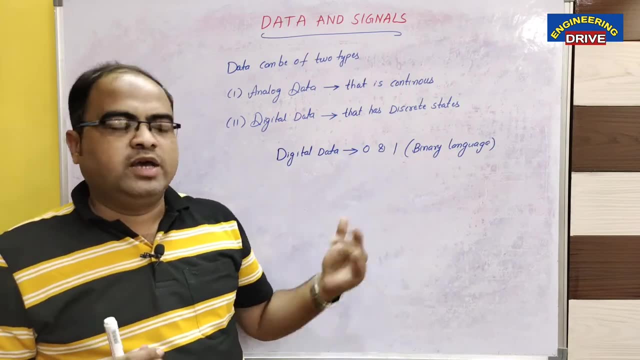 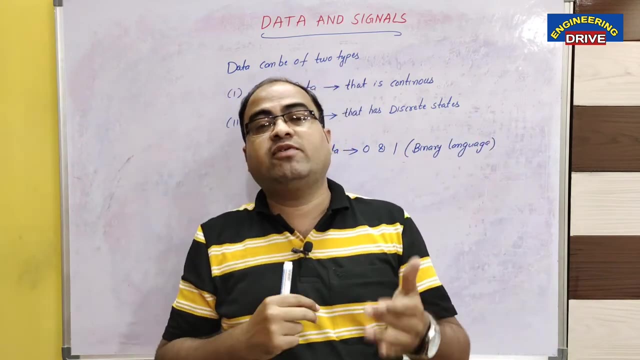 So, dear students, the point should be clear: that computer understands only digital data, that digital data will be available in zeros and ones. Now, in order to establish communication between one computer to another computer, what happened During the transmission? the data will be converted into analog signal and that data 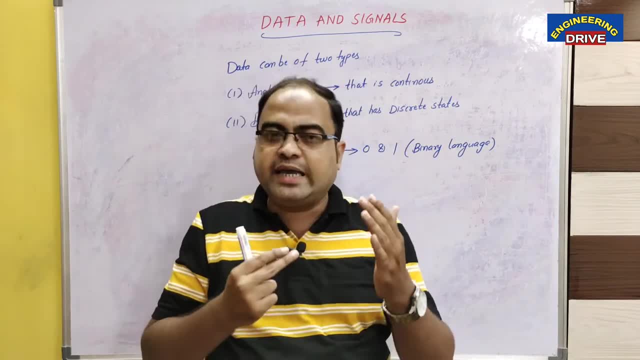 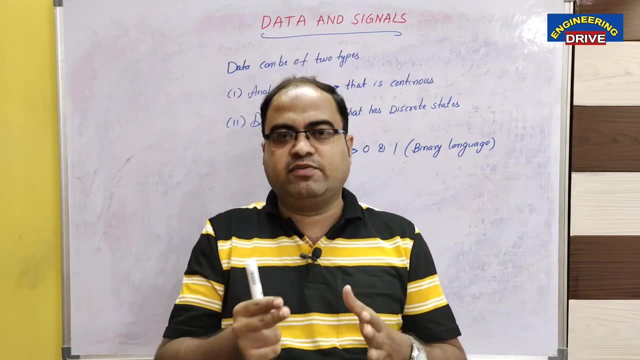 will be transmitted. Once the data will be received to the computer, again it will be converted back to digital form. So who will take care of this work? Modem modulator: demodulator: it is a device which converts this signals into vice versa. 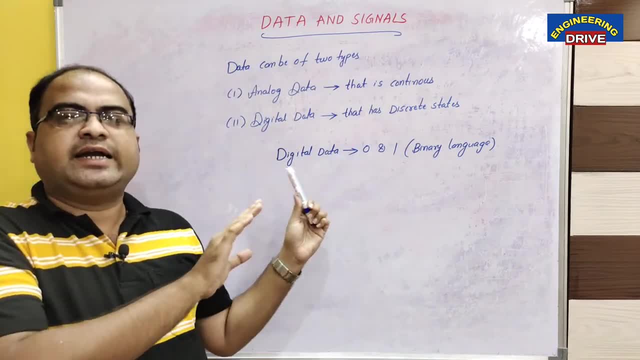 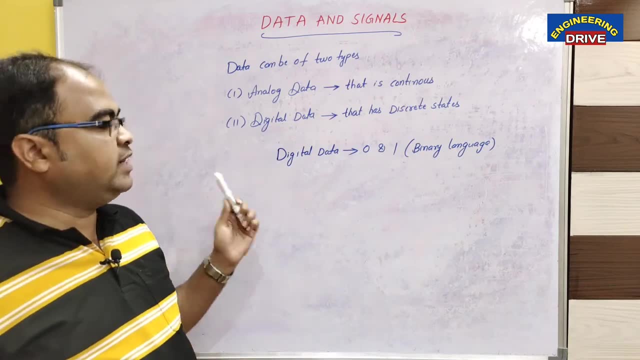 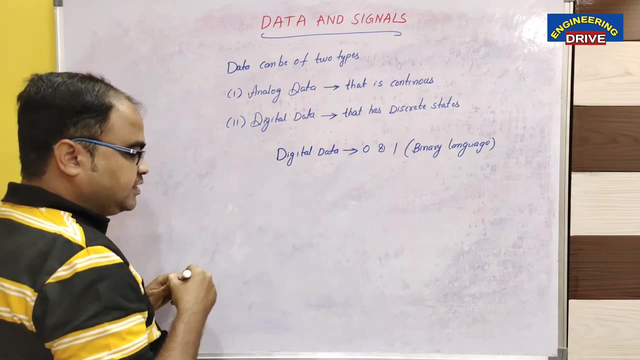 Is it clear? Now? this is about digital and analog data. Okay, Now, while coming to the signals, now let me show you graphically what is the difference between analog signal and digital signal. now, Now, in order to show the main difference between analog signal and digital signal. 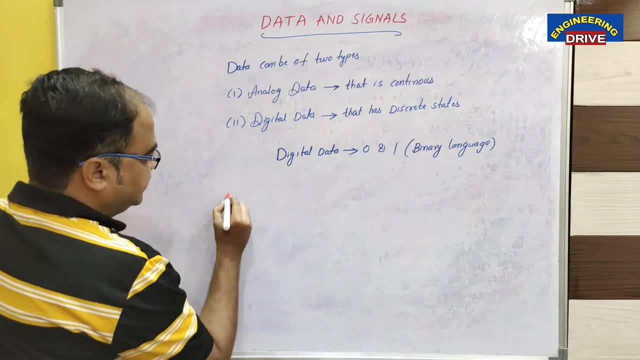 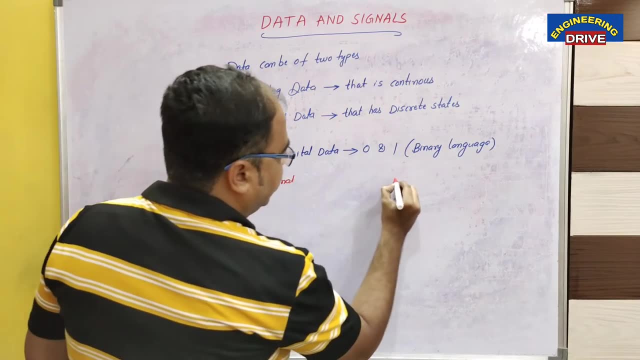 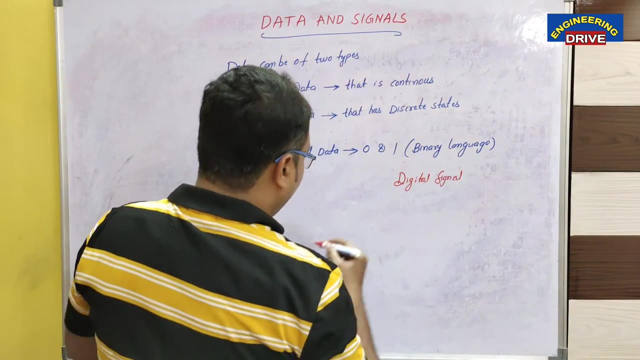 let me draw a perpendicular axis graph now. So let us take: this is a analog signal and this is, on the right hand side, digital signal, digital signal. Okay, Now let me show you here the difference between this. Let me draw a perpendicular axis now. 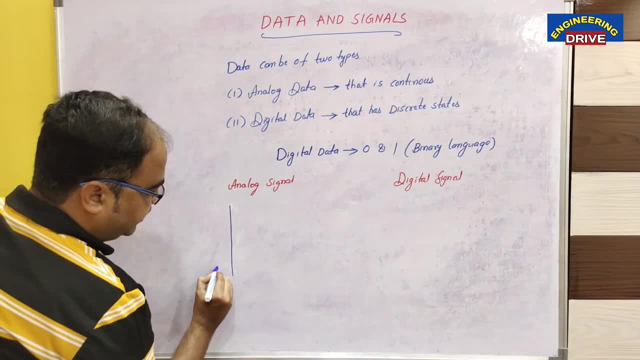 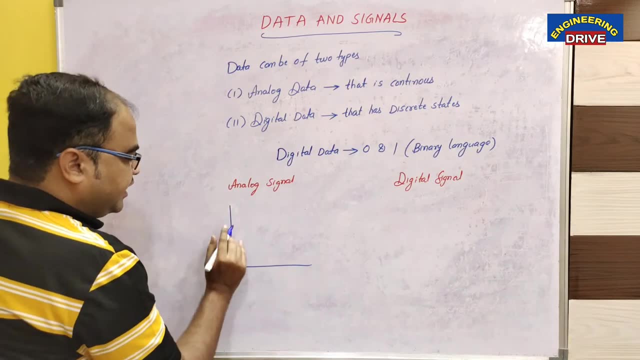 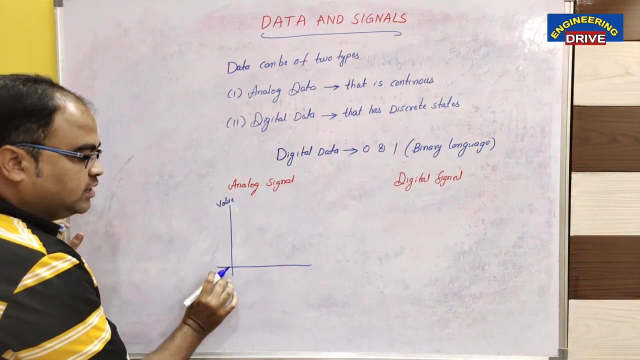 So this is one axis, that is vertical axis and this is horizontal axis. So this vertical axis, let us treat, let us take it as a signal value or strength of a signal. This is the vertical axis, Okay, Whereas the horizontal axis represents the signal. 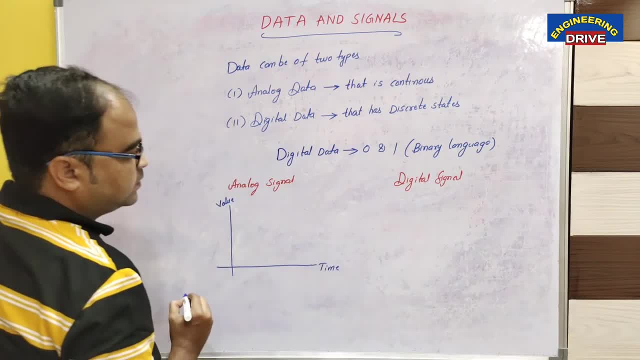 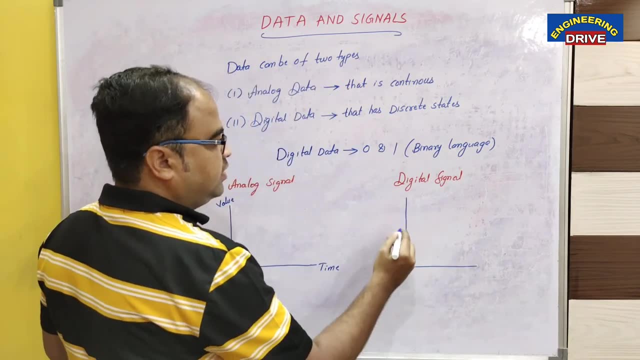 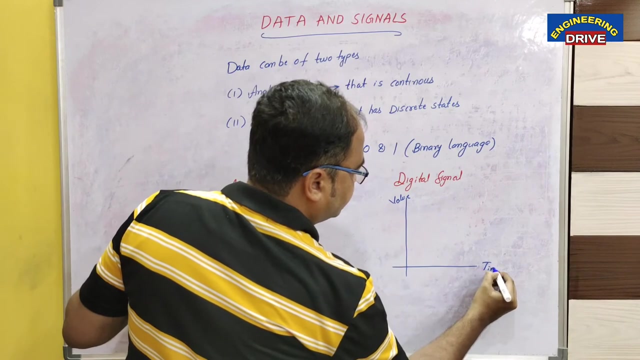 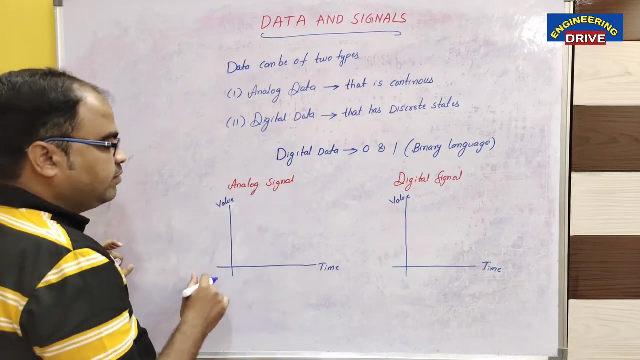 Okay, Similarly here also. Here also, we will take perpendicular axis, two perpendicular axis here. So here same. this is the signal value and here the time. Now, what about analog signal? how it will look like. So analog signal is nothing but which is continuous. 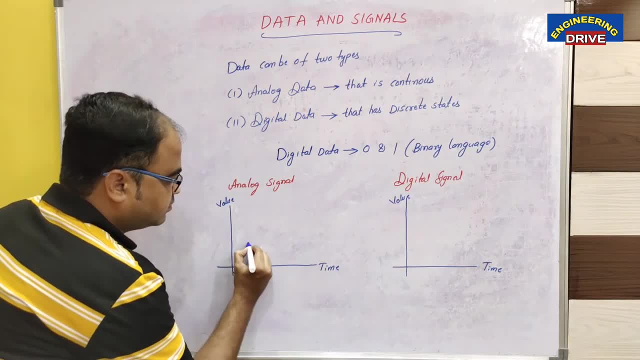 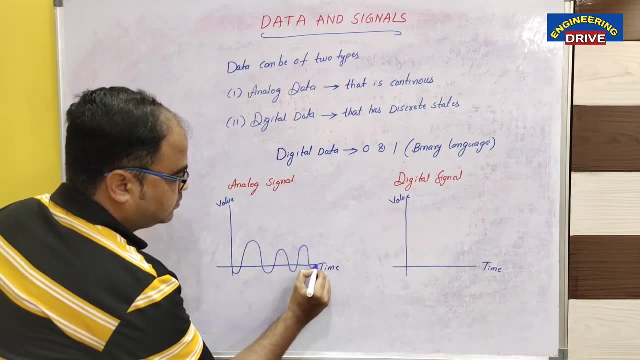 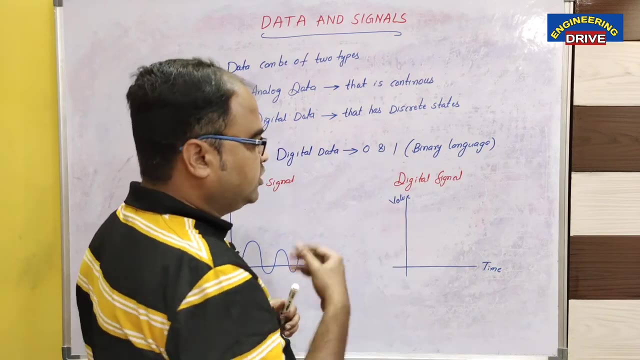 So what happened Here? you will get the wave in this manner, Something which is continuous. this is an analog signal, Whereas, on the other hand, digital signal is nothing but which is binary form- zeros and ones- and it is having discrete states.